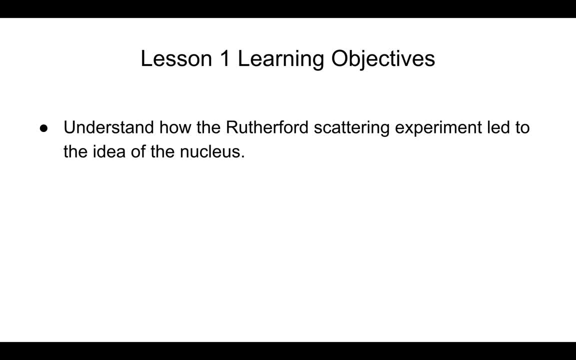 one, you will be able to understand how the Rutherford scattering experiment led to the idea of the nucleus. You will also be able to discuss how scattering experiments may be used to determine nuclear radii, And there will be, of course, some math involved here. So first let's discuss. 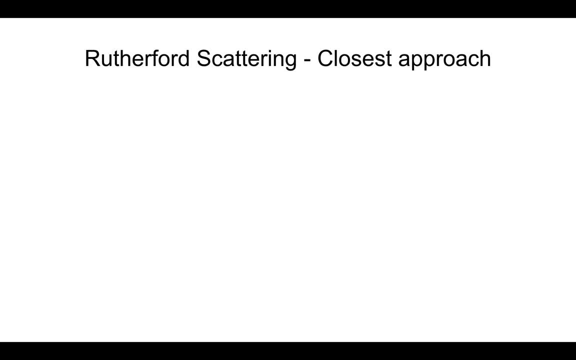 Rutherford scattering and this important idea of the closest approach. So you might recall the Geiger-Marston experiment from topic 7, where alpha particles are emitted from a radioactive source and blasted through a gold foil, And this resulted in the surprising experience that some of the 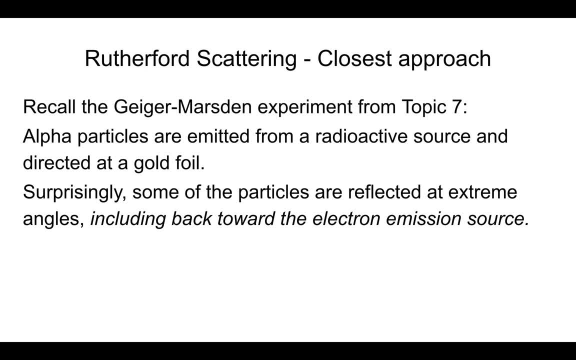 particles deflect or even reflect backward toward the emission source. So what they expected was a small-angle deflection, a slight deflection, and what they got was, in very rare instances, extreme deflection. Okay, so this surprising result suggests a small, dense nucleus at the heart of each atom. 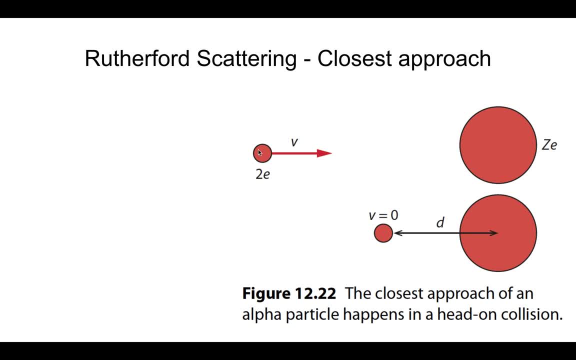 So here we have a diagram, And what we have here is an alpha particle approaching a nucleus, And you will recall that Z is the proton number of this nucleus. Okay, so the number of protons is given by Z, E, of course, is the fundamental charge. 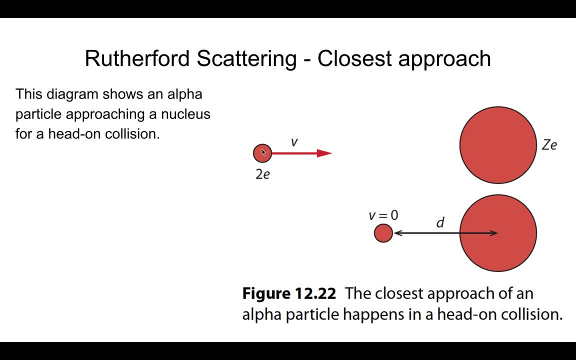 Okay, so this is the fundamental charge, And you will recall that Z is the proton number of this nucleus. Okay, what we have here, then, is a head-on collision, where our alpha particles headed toward the exact center of this nucleus, And this is going to produce the closest. 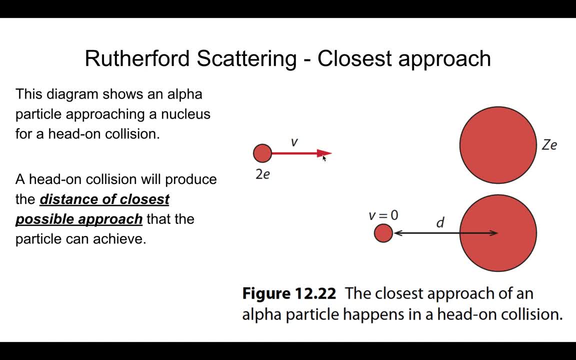 possible distance that this alpha particle can achieve in relation to the larger nucleus. Okay, so that's what we mean by distance of closest possible approach, And what's going to happen here is that the alpha part of alpha particles- kinetic energy, is converted then to electric potential. 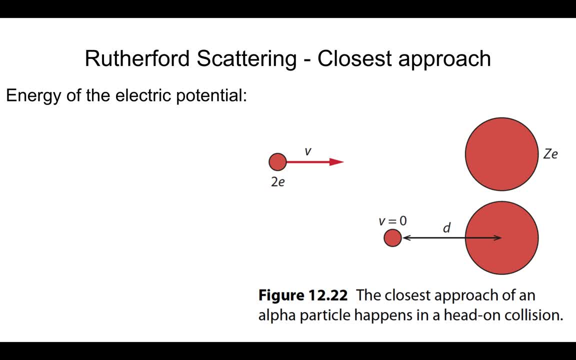 energy. So we know that the energy of electric potential is equal to Coulomb's constant times the charge of the larger object, or the larger charge times the smaller charge divided by the distance between the two objects. Okay, so we can further quantify that by incorporating our charges 2 times a fundamental charge. 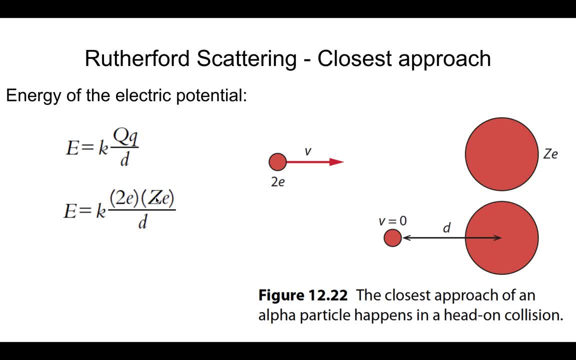 that is the charge of an alpha particle. Z again is the proton number multiplied by the fundamental charge of a proton divided by D. Note here that all of our charges are positive. We don't have any electrons involved in this interaction. Okay, we can then simplify. 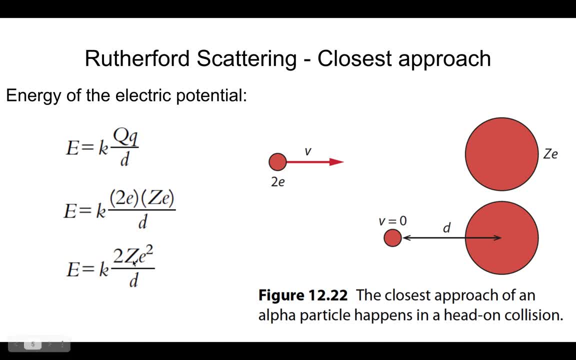 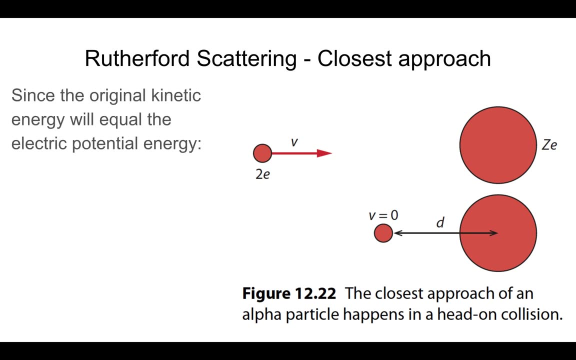 that to Coulomb's constant times, 2 times our proton number, times a fundamental charge squared divided by the distance between our two objects. for the closest possible approach, And since our original kinetic energy is going to equal that electric potential energy, that previous formula then will give us the kinetic energy of our alpha. 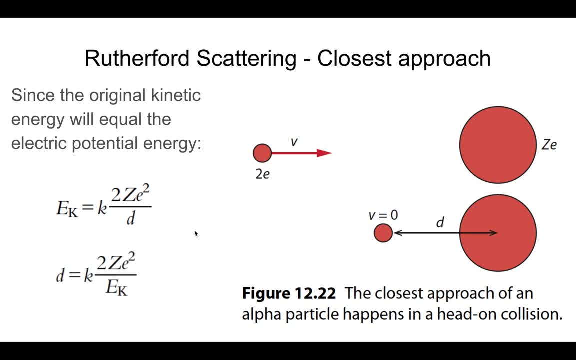 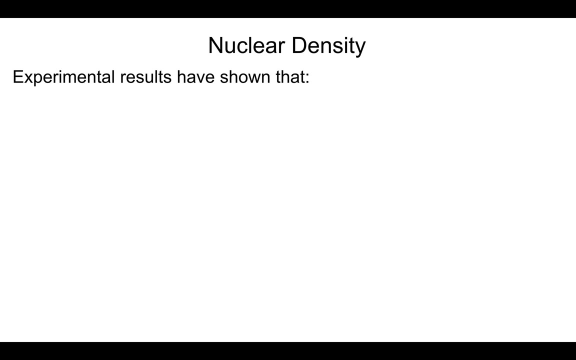 particle on its closest possible approach, And we can solve that equation then for the distance of the closest possible approach, and that looks like this: I don't need, I think, to redefine these variables. This, of course, is kinetic energy. Okay, so experimental results have shown that r is equal to r sub 0 times a to the. 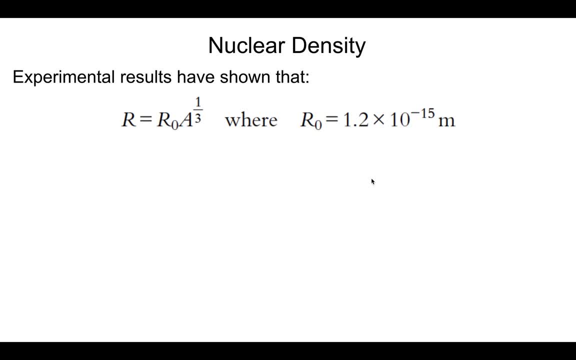 one-third power, And of course this is completely meaningless until we define our variables. So let's do that. R is the nuclear radius, A is the atomic mass number- Okay, important that we don't confuse that with the proton number- And r sub 0 is what we called the Fermi radius, which we should further define. 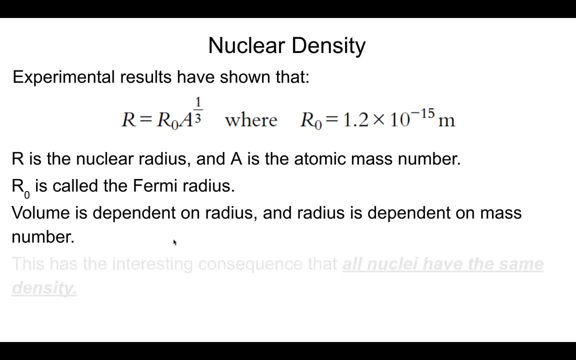 Volume is dependent on radius and radius is dependent on mass number and consequently all nuclei have the same density Interesting, okay, r sub 0 or Fermi radius- just to make sure we're clear on this- is defined as 1.2 times the surface. 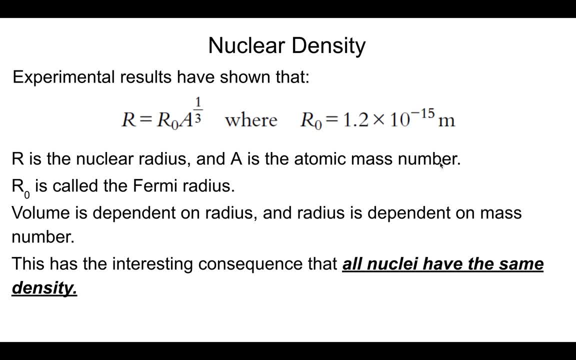 times 10 to the negative 15 meters. Okay, so we've established, then, that all nuclei have the same density, and if you'd like to further explore the math, your SOCOS textbook shows it an example: 12.14. so go ahead and check it out if 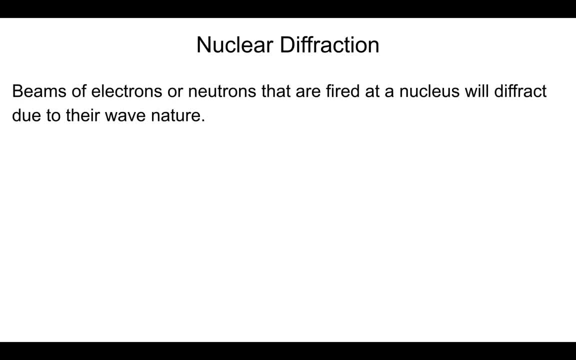 you're curious, Okay. so, as we discussed in topic 12.1, objects with mass have wave behavior as well. What that means is that if we shoot electrons in a nucleus, they will diffract, just like you would see diffraction around any other. 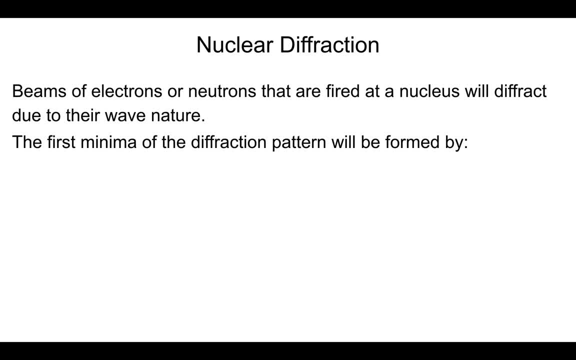 object. So we can find the first minima of the diffraction pattern by taking the angle to the minima and approximating it, the sign of that angle. by taking the angle to the minima and approximating it, the sign of that angle. 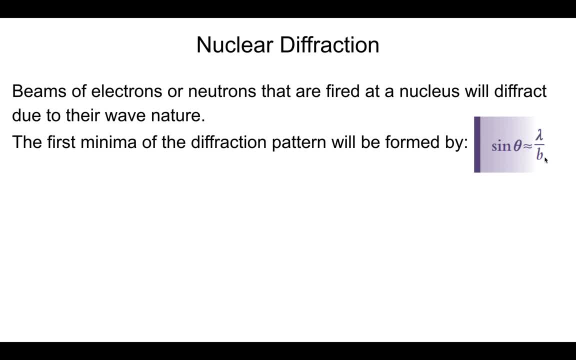 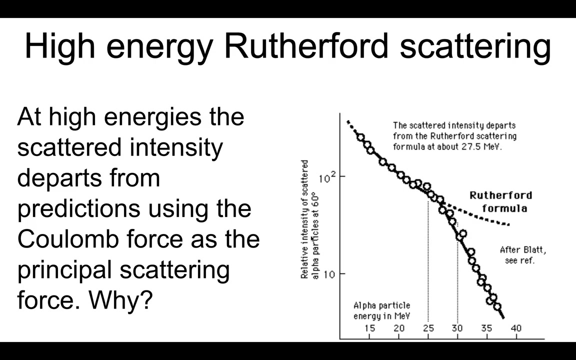 approximating the sign of that angle to the wavelength divided by B. and again we need to define our variables. B is the diameter of the nucleus and lambda is our de Broglie wavelength. So there you go. Okay, so where we have high energies, the scattering intensity is: 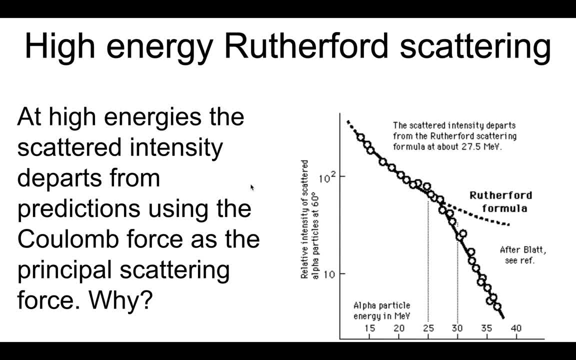 the same as the scattering intensity. So we can see that the scattering intensity departs from predictions using Coulomb force as our principal scattering force. So you can see it here. So there's this point where we just diverge from Coulombic force. So what's going on here? Go ahead and think it over and if you're with a 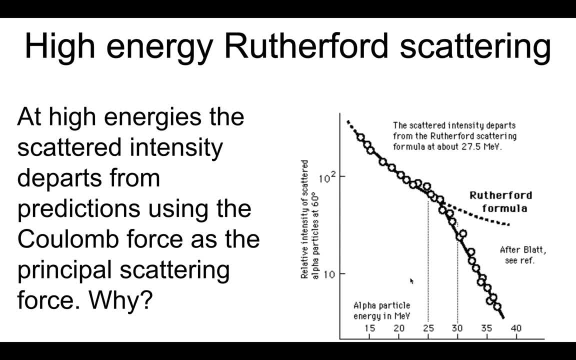 friend or two, you may wish to discuss it. Why is this happening? What's going on? Why? So we're blasting- just to reiterate, we're blasting- alpha particles at a nucleus and we're increasing the kinetic energy of that electron, in other words, or alpha particle, rather, in other 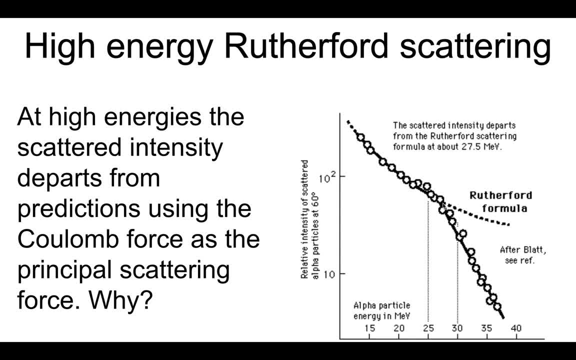 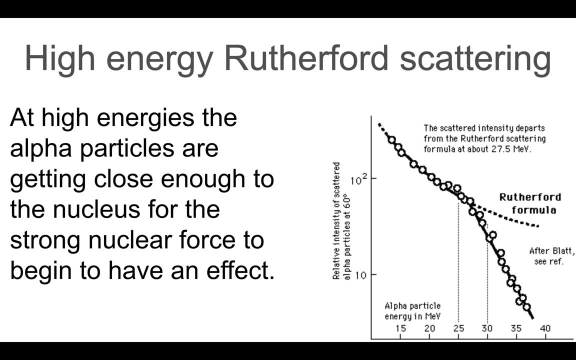 words, increasing its velocity until we get to this point where our behavior changes. So what's happening? Pause, Okay, I assume you have thought it over And I assume that you have correctly predicted that our alpha particles have enough kinetic energy that they can get closer to the nucleus. 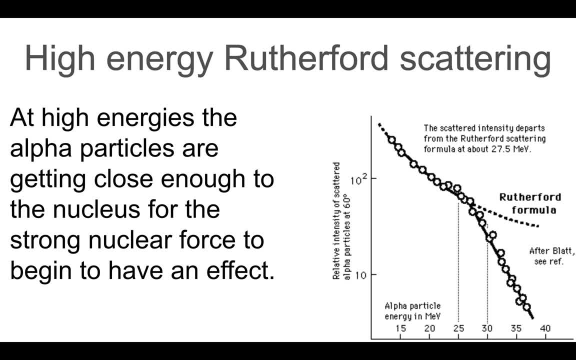 Remember that they are repulsed because they're both positively charged, So they don't want to get close to each other. But if it has enough kinetic energy, what happens is that strong nuclear force will begin to take over. Remember that strong nuclear force is only effective at a very, very, very short distance. 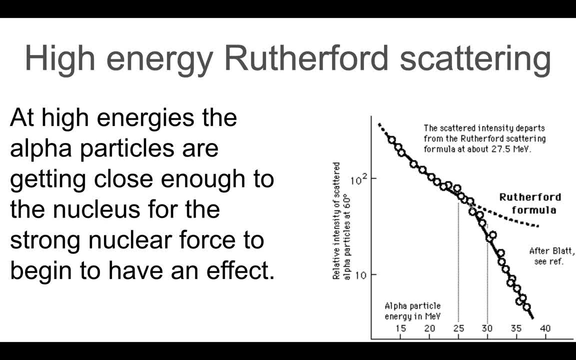 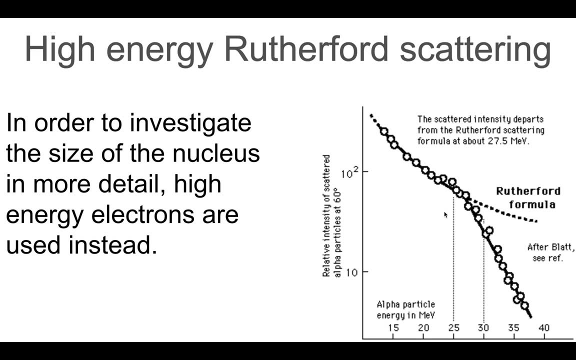 And if our alpha particle has enough kinetic energy, it can get within that radius where strong nuclear force begins to have an effect And that changes the behavior of our alpha particle. Okay, so if we want to investigate the size of the nucleus, we use high energy electrons. 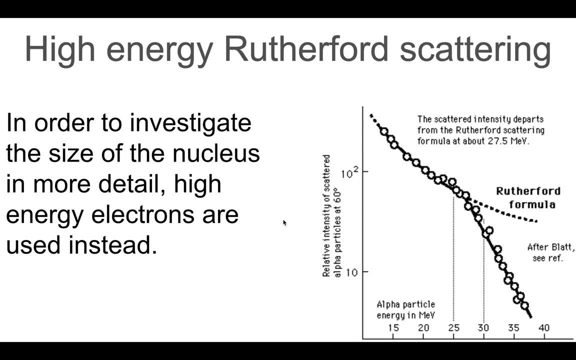 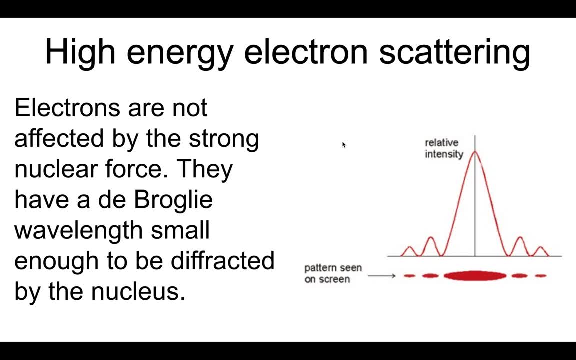 Instead of alpha particles. The reason for that is because electrons aren't affected by strong nuclear force And they have a very, very tiny de Broglie wavelength And it is small enough that it will be diffracted by our tiny, tiny nucleus. 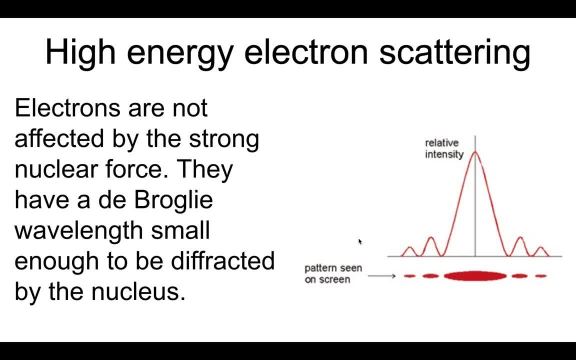 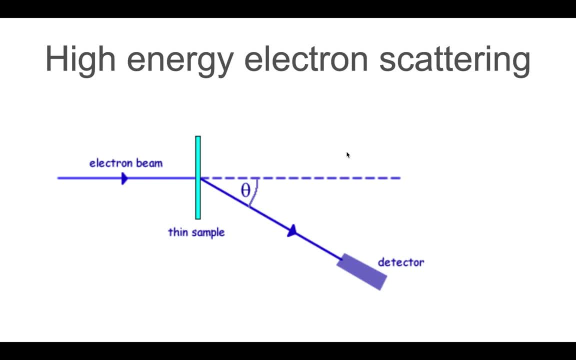 And that diffraction is going to produce, of course, a diffraction pattern, Which you will realize, If you recall, from Topics 4 and Topic 9.. Okay, and this is just a reminder of what our scattering looks like, We have an electron beam. 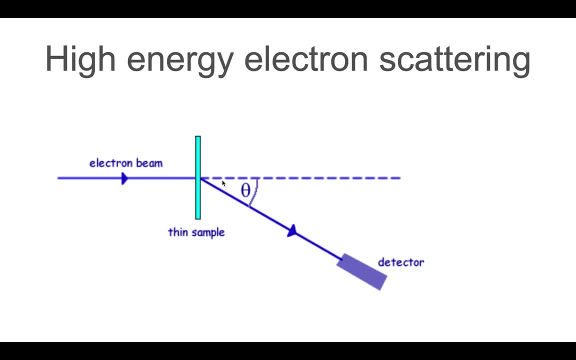 And this looks a lot like the Marsden experiment, where you have a detector that is rotated around, a sample, Okay, and it is picking up electrons, And the angle then is measured. Okay, so we are going to find that our electron beam is diffracted.